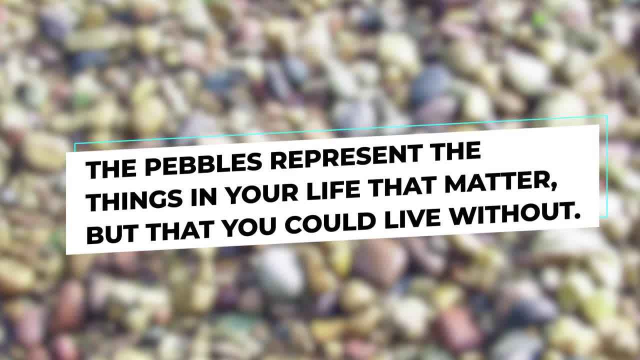 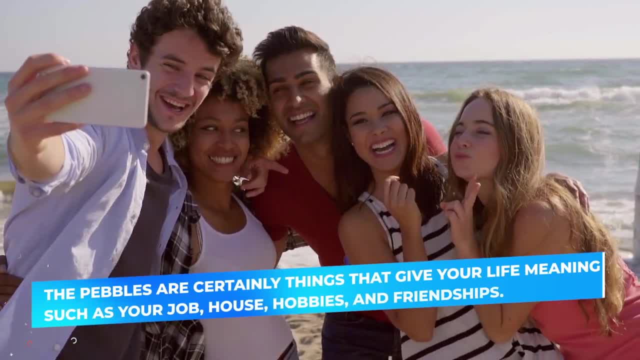 The pebbles represent the things in your life that matter but that you could live without. The pebbles are certainly things that give your life meaning, such as your job, house, hobbies and friendships. They are not critical for you to have a meaningful life. 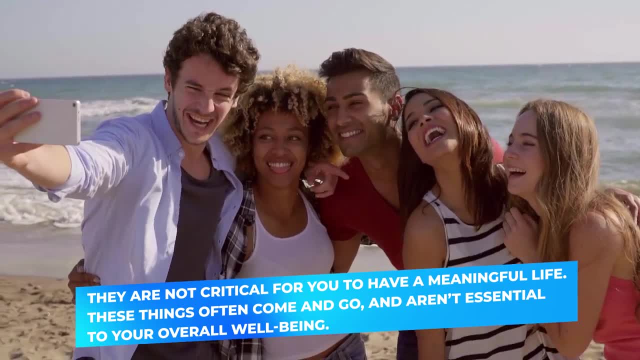 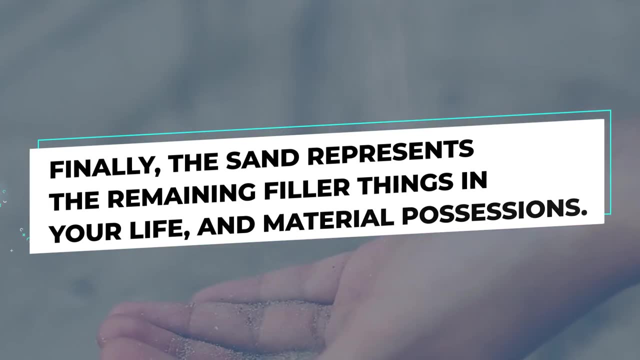 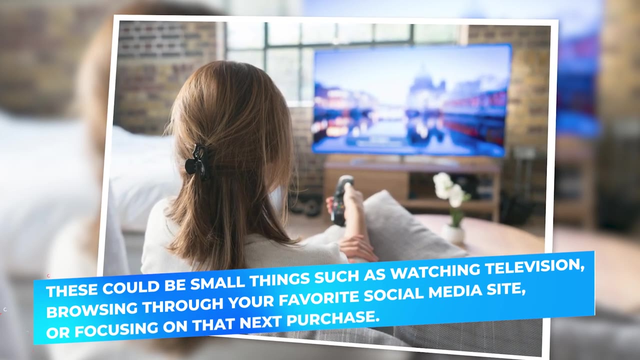 These things often come and go and aren't essential to your overall well-being. Finally, the sand represents the remaining filler things in your life and material possessions. These could be small things such as watching television, browsing through your favorite social media site or focusing on that next purchase. These things don't mean much to. 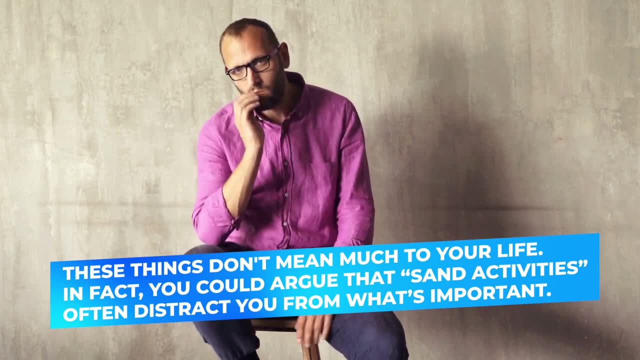 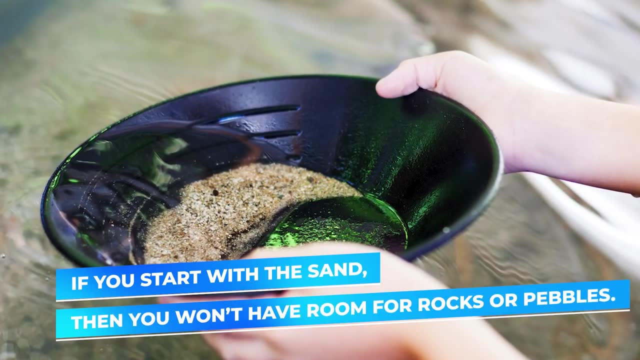 your life. In fact, you could argue that sand activities often distract you from what's important. If you start with the sand, then you won't have room for the rocks and pebbles. This holds true with the things you let into your life. If you spend all your time on these small 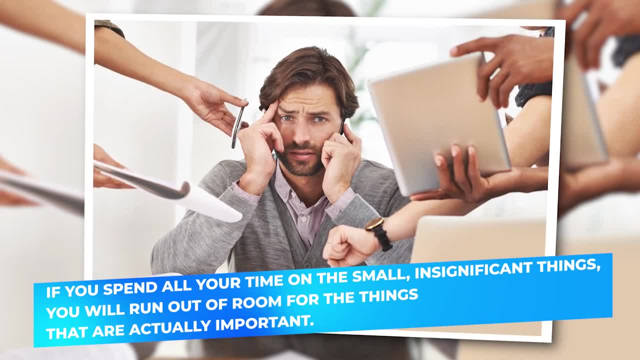 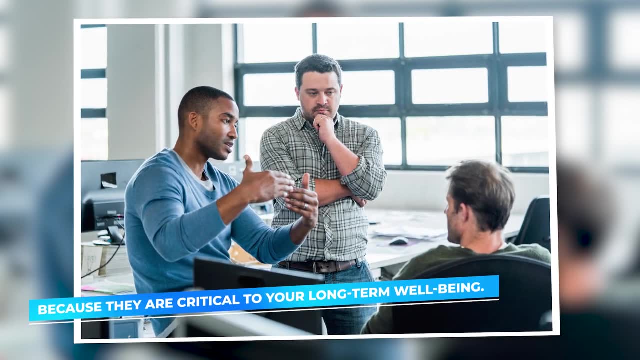 insignificant things, you'll run out of room for the things that are actually important In order to have a more effective and efficient life. pay attention to the rocks, because they are critical to your long-term well-being. These rocks can include building a career that is personally rewarding. 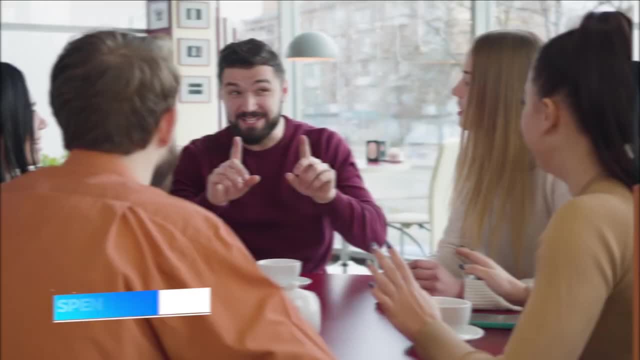 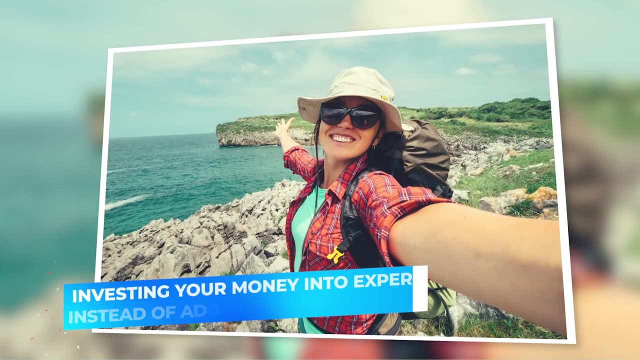 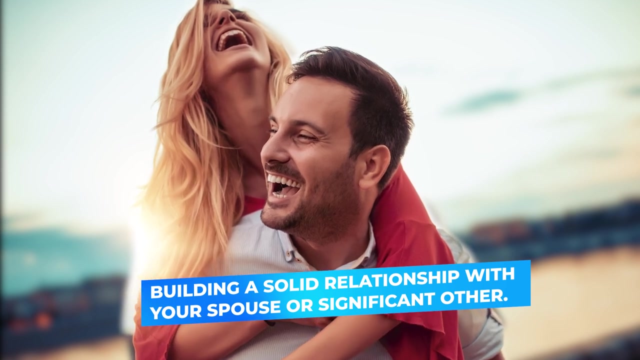 paying close attention to your health. spending time with your family and loved ones, enjoying hobbies that add value to your life. investing your money into experiences instead of adding another possession, building a solid relationship with your spouse or significant other. While you can always find, 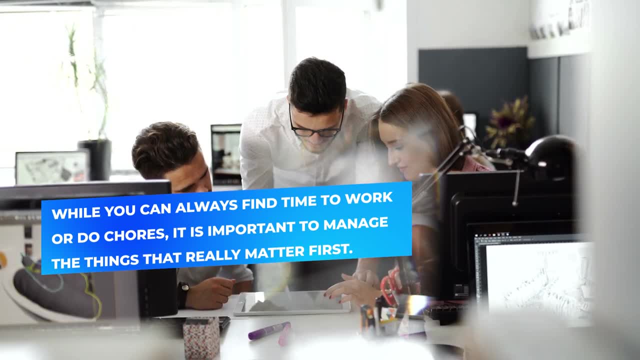 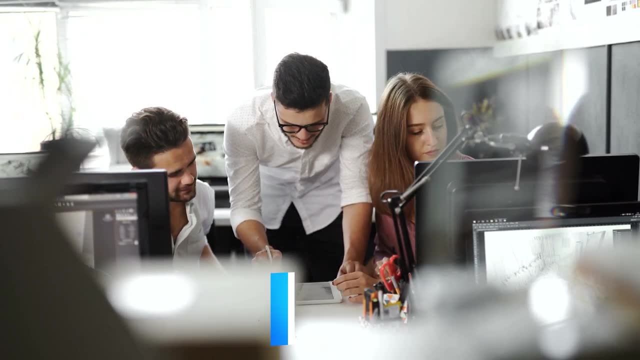 time to work or do chores. it's important to manage the things that really matter first. The rocks are your priorities, while the other things in your life are represented by pebbles and sand. So to focus on what's important, it's best to have a maximum of five rocks in the jar. 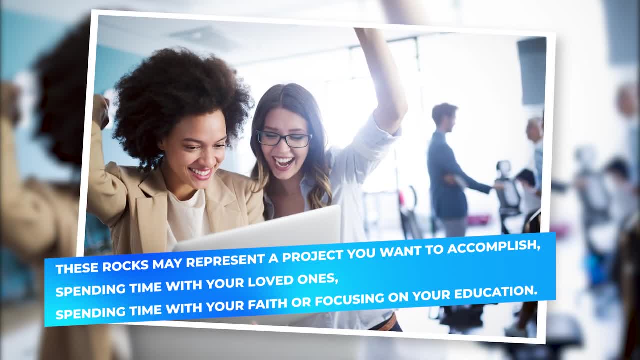 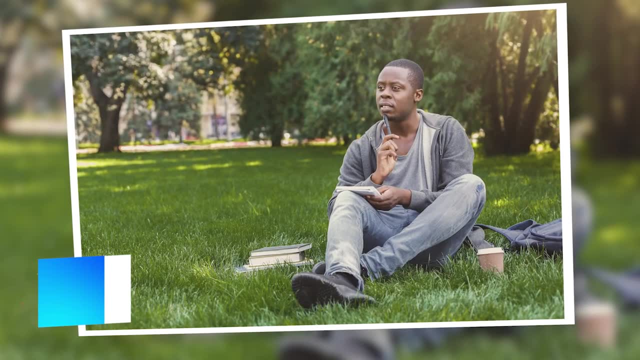 at any given time. These rocks may represent a project you want to accomplish: spending time with your loved ones, spending time with your faith or focusing on your education. The big lesson here is: if you're able to identify the rocks that matter to you, then you're going to. 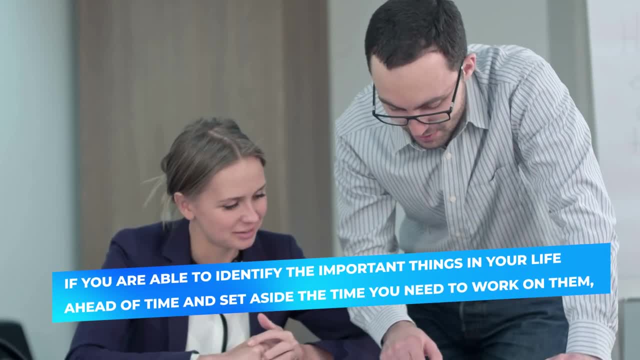 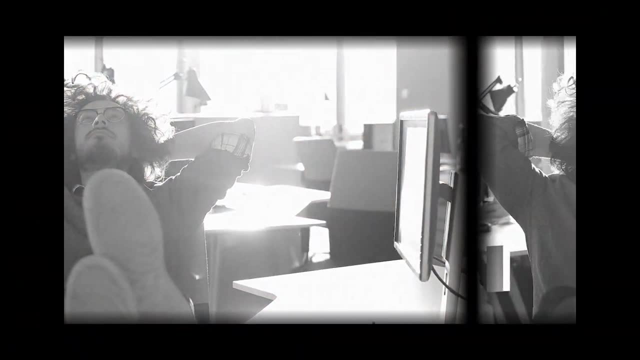 be able to work on them. If you can identify the important things in your life ahead of time and set aside the time you need to work on them, then it's okay to procrastinate a bit on the pebbles or the sand tasks that aren't as important. Finally, if you'd like to see more actionable,